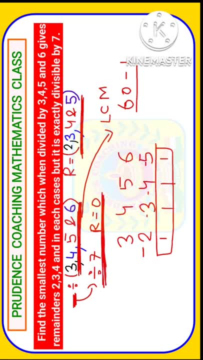 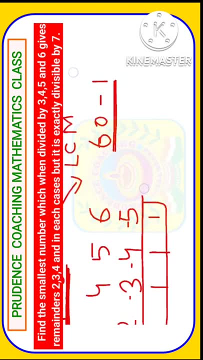 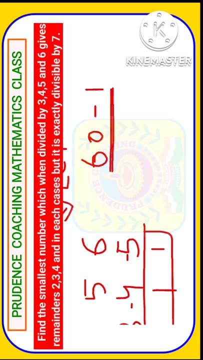 But along with that in this question another one, Freq, is there, that is, this number must be completely divisible by 7.. So here, 60-1 is not divisible by 7. So 60-1 is 59,, 59 is not divisible by 7.. 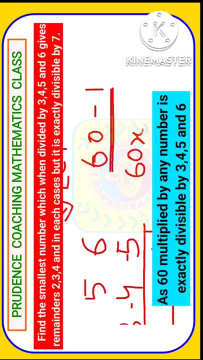 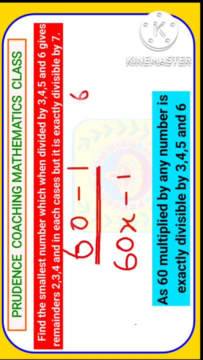 So we will put a x beside the LCM, then minus 1. we are going to add Now the LCM, that is 60x. we will divide 60 by 7.. As this number is exactly divisible, Divisible by 7.. 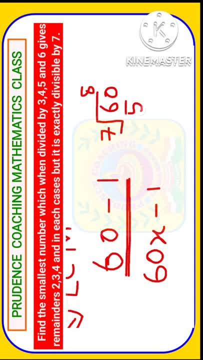 So here you will get 7,, 8,, 0, 56.. So remainder, you are getting here 4.. That means from 60, if we deduct 4, then that number, that is 60-4, 56, is completely divisible by 7.. 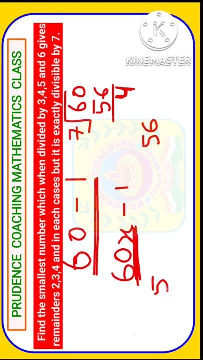 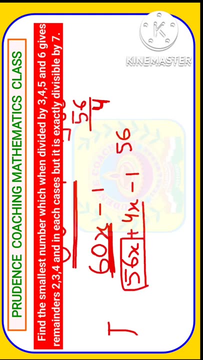 So if we just write this as 56x plus 4x minus 1.. So here 60x is written as 56. Here 56x is completely divisible by 7. So we need not to worry about that. Here 4x minus 1 is not divisible by 7.. 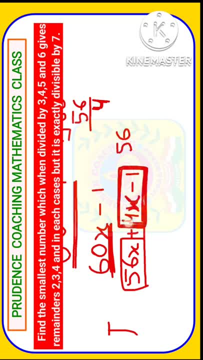 So we need to assume a value of x such that number is divisible by 7. So if we assume it 1, then 4 into 1 is 4 minus 1. You will get 3. So 1 is not the value. 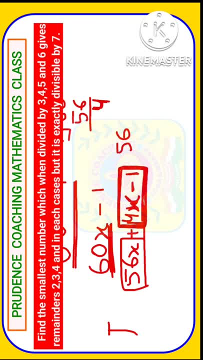 If we take 2, 4,, 2 are 8.. 8 minus 1 is 7.. So 7 is divisible by 7.. That means here x is equal to 2.. So put x equal to 2 here. 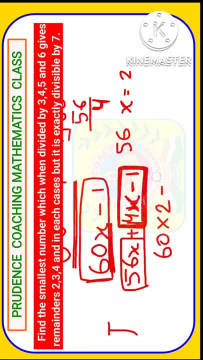 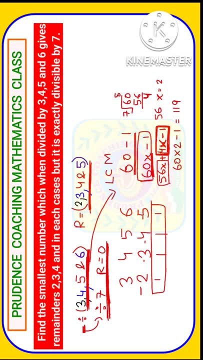 So you will get 60 into 2. That is 120 minus 1. You will get here 119.. So here 119 is our answer.